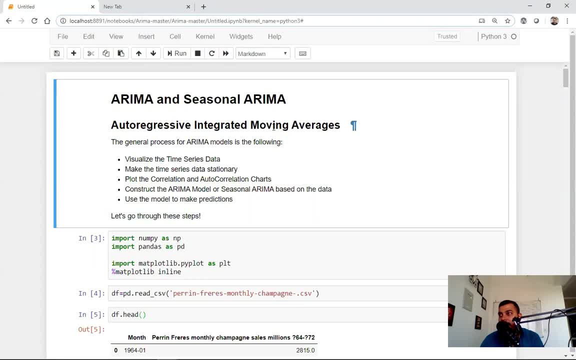 is auto-regressive, then we have integrated, then we have moving averages, And auto-regressive formula is a little bit different. moving average formula is a little bit different, And we'll also try to understand what this integrated value says. This is also called: 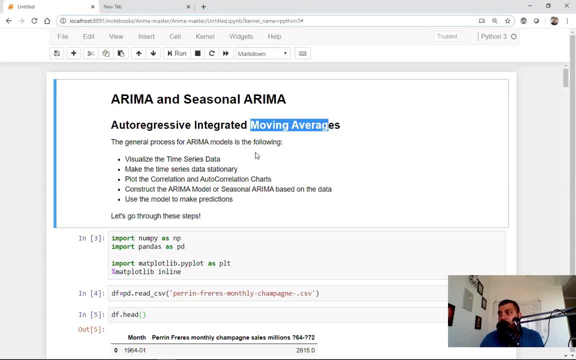 as differencing. Now our general process for ARIMA model is something like this: First of all, we'll visualize the time series data. We'll try to check out whether the time series data is stationary. If it is not stationary, we'll try to make it as stationary. Then we'll try to plot the 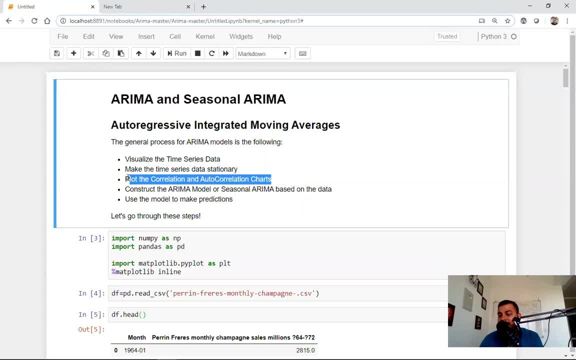 correlation or autocorrelation charts, because this will help us to tell us what will be the lags value in case of auto-regressive and moving averages. Remember, in auto-regressive, whenever we are implementing it. I'm going to show you the formula just in a while There. 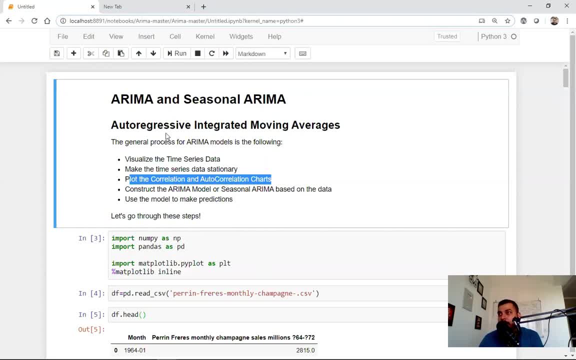 there are some values, which is also called as lags. So suppose your today output is y and it is actually dependent on some data of the previous day. Okay, So suppose if I want to predict today's sales data, so it may be dependent on past three days, right? 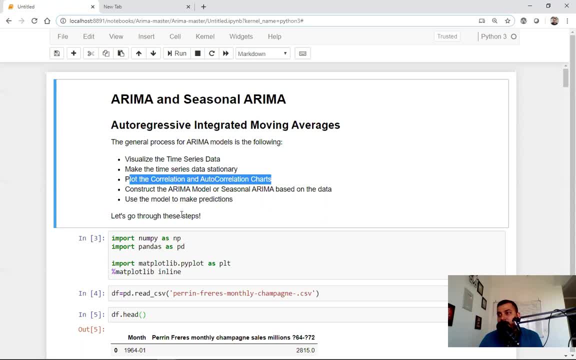 So past three days is my lags, So those kinds of values it will help us to select. Then we'll try to construct the ARIMA or the seasonal ARIMA model based on the data. I'll tell you when to select ARIMA model, when to select a seasonal model, and then we'll try to make. 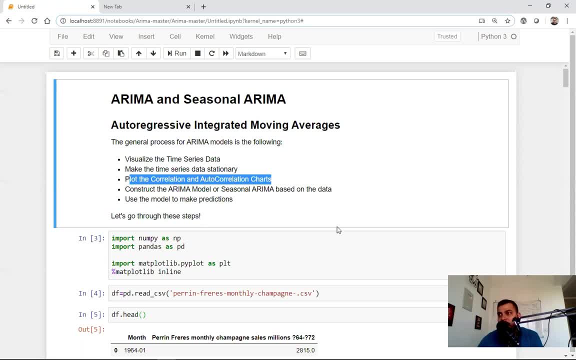 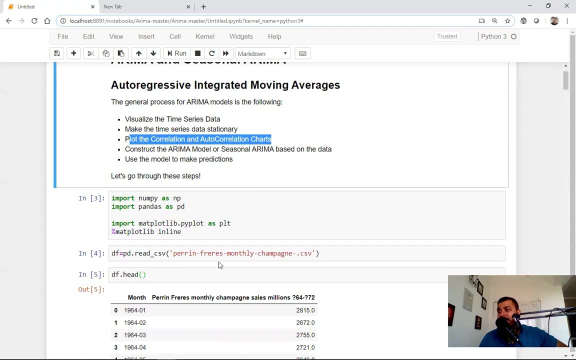 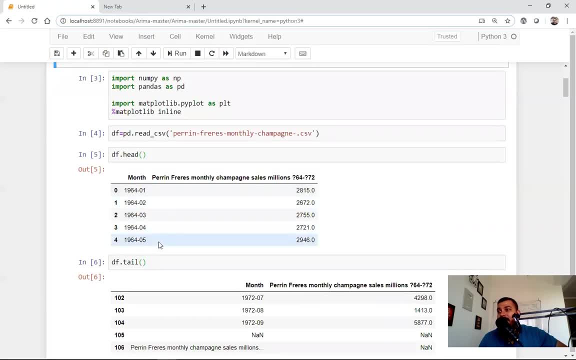 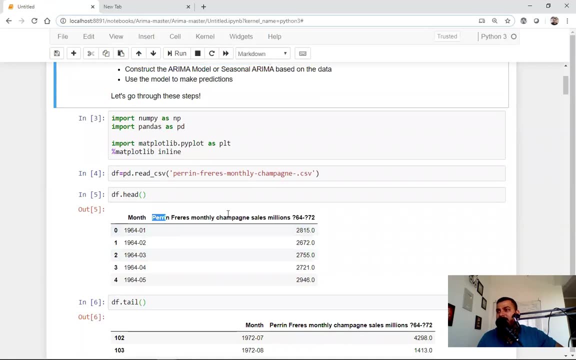 produced. in short, and this, the data is basically from 1964 to 1972. so, first of all, what I had observed, and this particular data set is available freely. you can actually get it from Kaggle, you can get it from some other sites also. anyhow, in my github you'll be able to find out all the materials, along with 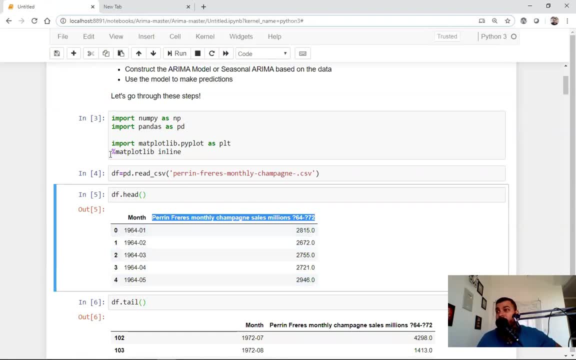 the data set. so, to begin with, what we are going to do is that we are going to read this particular data set and we are going to see the head. in the head we can see the column name does not look good, so we are going to first of all change. 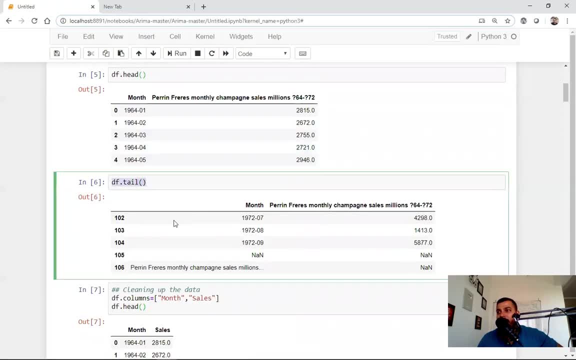 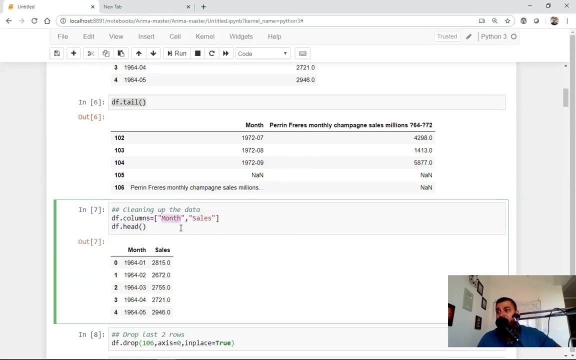 the column name. one more thing that we observed in dftail is basically two records were there which we had actually man values at the last records. okay, so we are going to remove these two records also. so here you can see. first of all I'm changing the column name so that it looks good. so I have changed it to month. 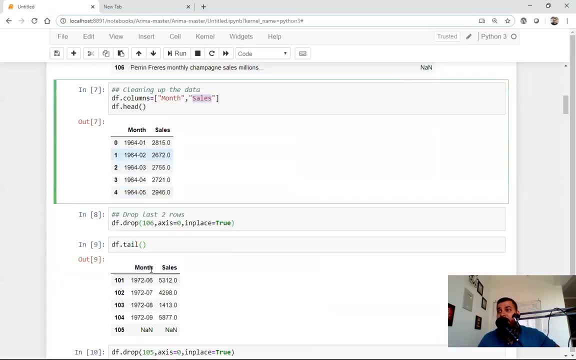 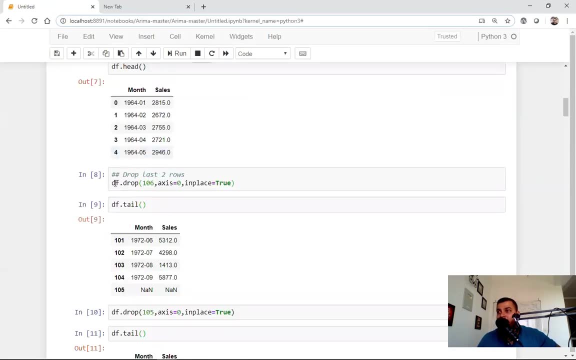 and sales. and I'm just seeing dfhead. you can see over here. right after that I'm dropping these two records. one is one zero five, one zero six. the first I'll drop. one zero six. for dropping you can just write dfdrop or you can give the index number of your row. then you're saying axis equal to zero. 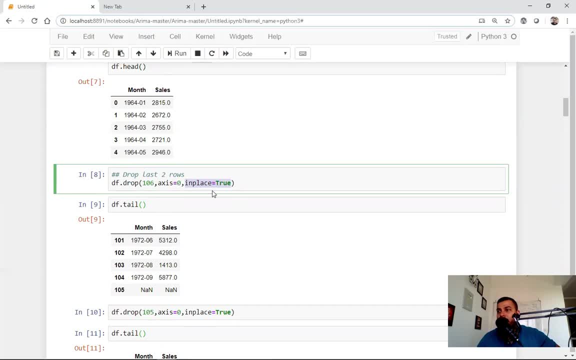 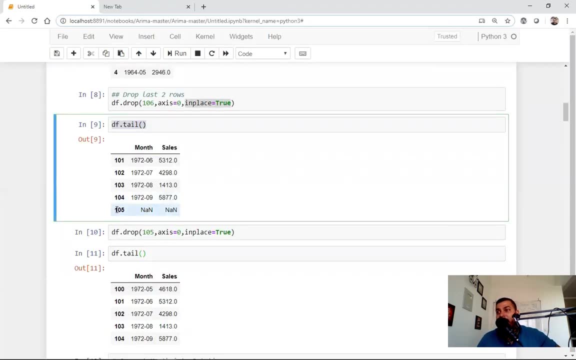 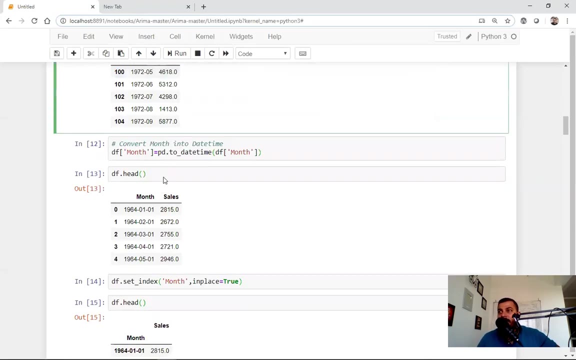 in place is equal to true, so it is an place operation, automatically the record will get deleted and to be stored there. then I'm going to check again dftail and I just have one man record and for that also I'm actually dropping it. so pretty much simple till here. now observe over here, guys. so we have data. 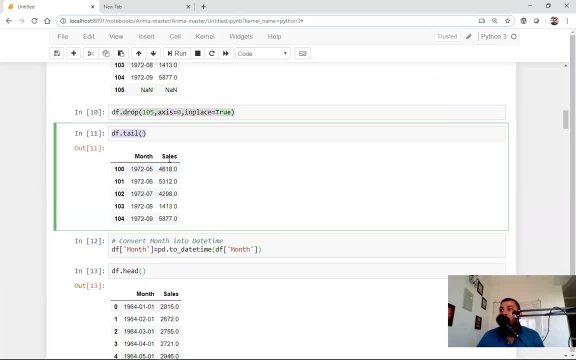 sets. observe the data set, guys over here we have a month column and sales column, okay, and if I try to see the type of this particular month, it is actually in the form of string format. so what we are going to do is that- so what we are going to do is that we are going to 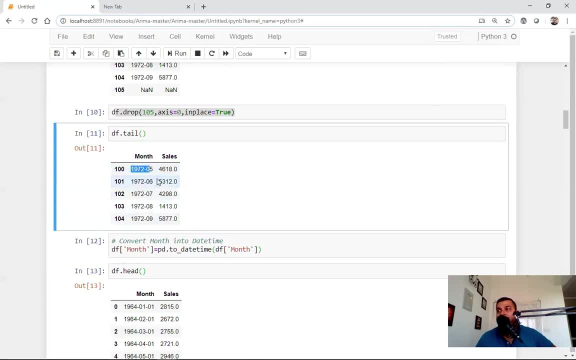 actually convert this whole month into date time variables, because it would be actually good for us because whenever we are working with time series, kind of data, at that time, specifically with respect to Arima and Seasonal Arima, at that time that we have to make that column as D. 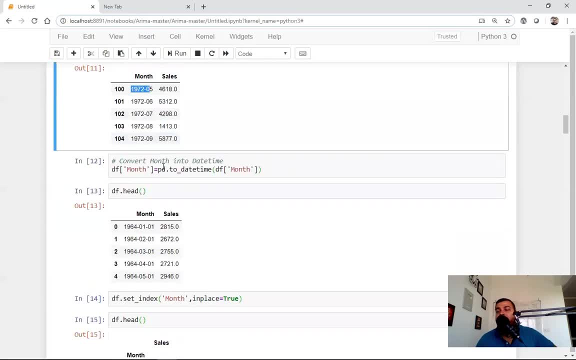 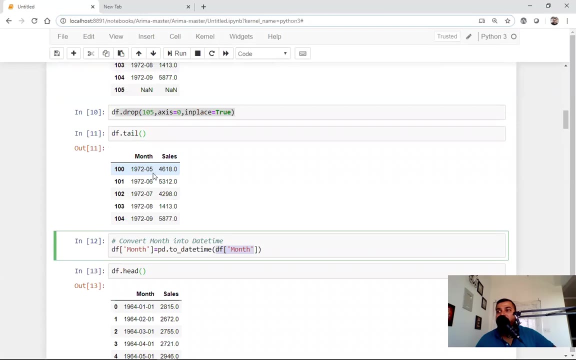 date time. So in order to make that date time, I have already imported Pandas library. So I am going to say pd.2, underscore date time, and here we have df of month. Now, when I do this automatically, you can see that when my data was something like this: 1972.05, this, 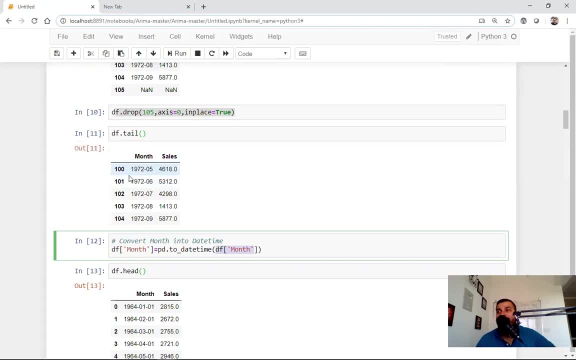 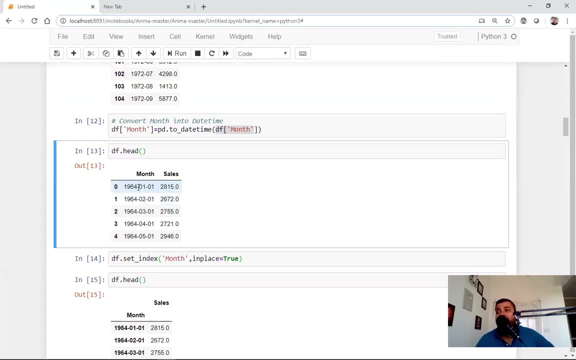 basically says that April month, not April May month, 1972.. So we are going to add in this particular format: now you can see that we have 01.01.1964. that basically says that first of Jan of 1964, first of Feb of 1964. So like this the data is actually present. 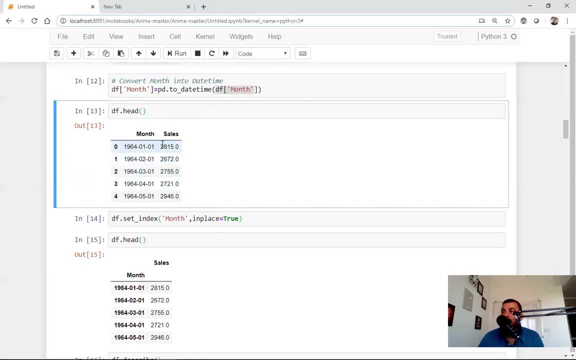 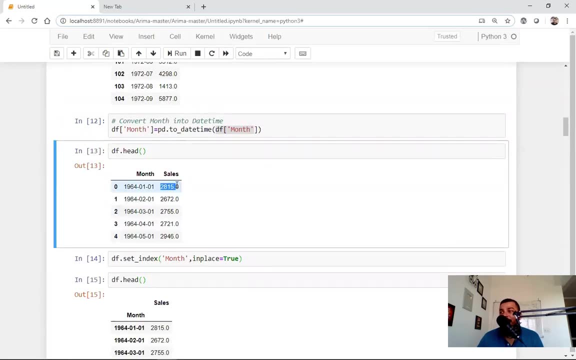 One more thing that you note about this particular data, guys, we have monthly data, So this sales. one thing that I forgot to say is that, guys, this is the sales of the champagne. I told the production of the champagne how much it was, So this was the sales average sales. 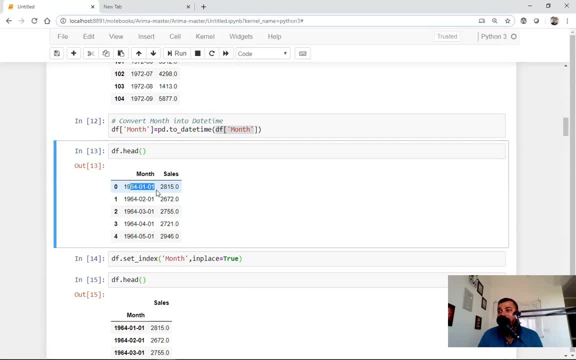 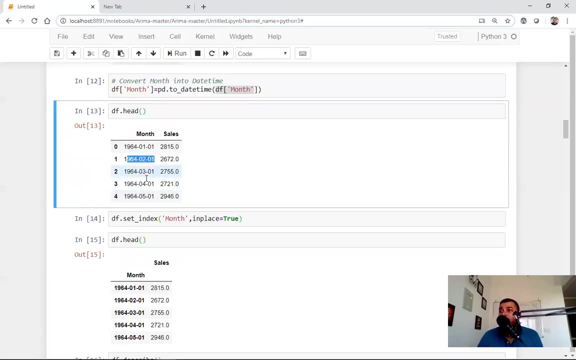 monthly average sales. So this month this was the sales. this month this was the sales. So we have actually monthly average sales data. Now, after doing this, I am going to quickly set this month column as my index. So for that I am just going to say dfset- underscore. 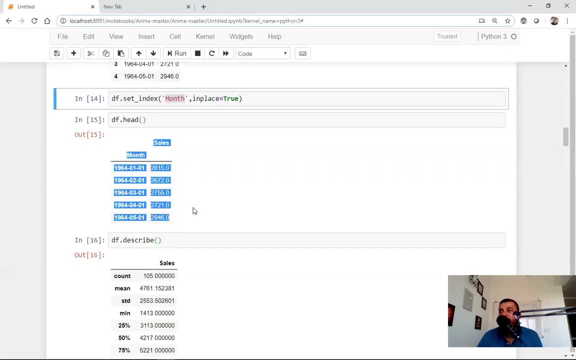 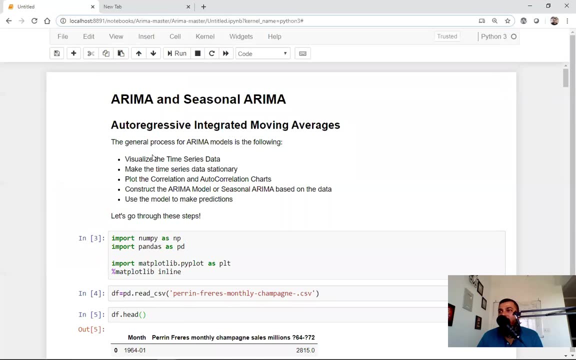 index month in place is equal to 2.. Now if I go and see my dfhead, you will be able to see the value like this. So pretty much simple. till here. What we have done is that we are just trying to visualize the time series data. we tried to see any nan values were. 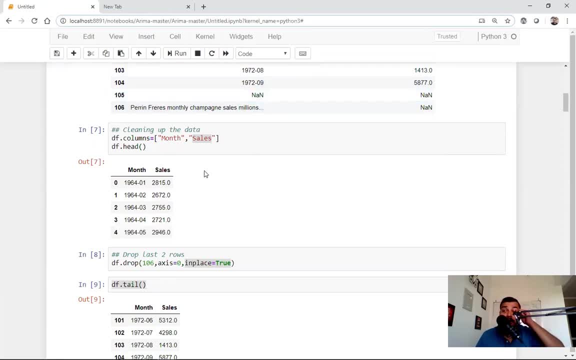 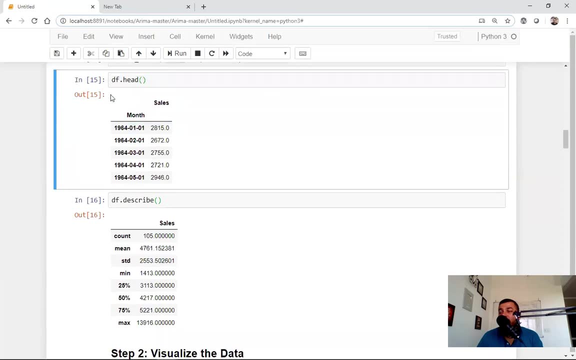 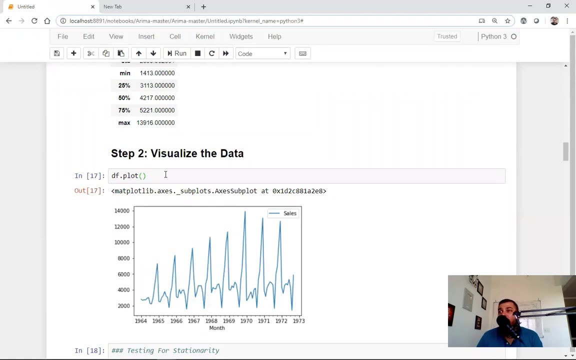 there we fixed it, And then we converted the month column into a date time column and then we finally set this as an index. So here is my the whole data with month as the index. Now step 2, visualization of the data. Now, first of all, 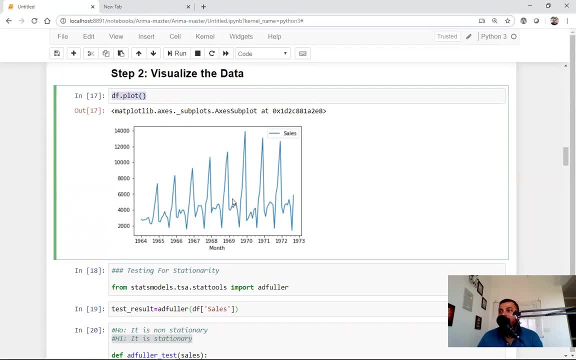 what I am going to do is that I am just going to say dfplot. Now here you can see all the data is over here and one thing that you note from this particular data. so what we are going to do is that, if you want to test whether this data is stationary or not, if you want, 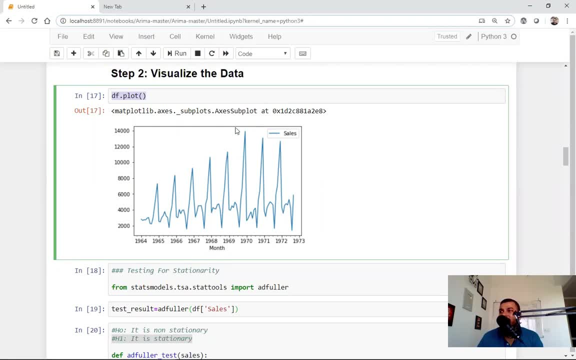 to test whether this data is stationary or not. and by just seeing this particular data guys, this data looks seasonal With respect to the year. Now what does seasonal mean? Understand that I have some sales data of ac selling of a particular company. Then 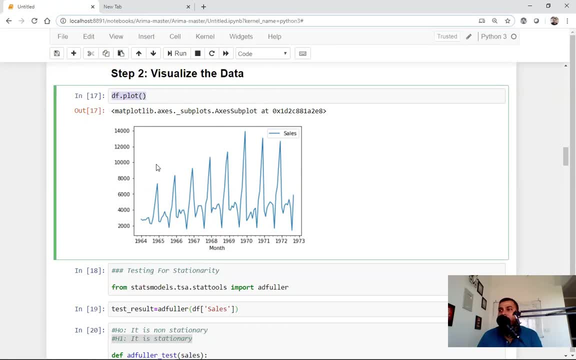 the data will look like: in the summers this AC is getting sold more. in the winters, the AC is getting sold less. So this is a kind of seasonal data And this may not be stationary right now, but it has some seasonal format. You know the data. 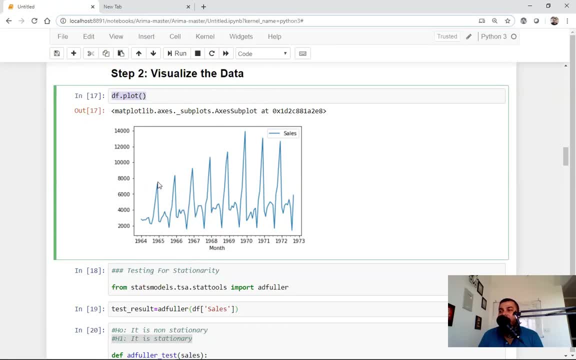 basically looks seasonal. okay, at some specific point of time the data is high, then the sales is high, then the sales is less. so these are kind of a seasonal data and it may- it may not be stationary. but our second step is that we have to check whether, how, whether the data is stationary or not, and if it is not, 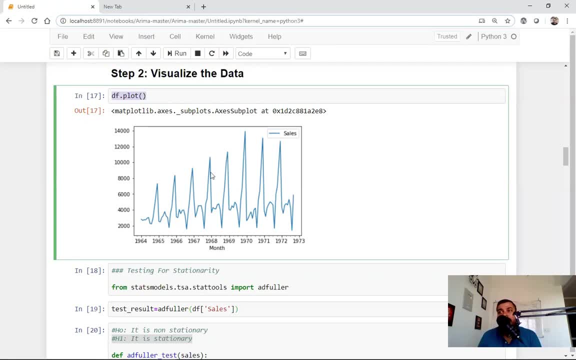 stationary. how do we make this a stationary? okay, two things, guys over here again. I'm telling you: this data looks seasonal. just by visualizing, you will be able to see that it is seasonal. now, in order to make the, in order to check whether a data is stationary or not, not only by seeing the mean and the. 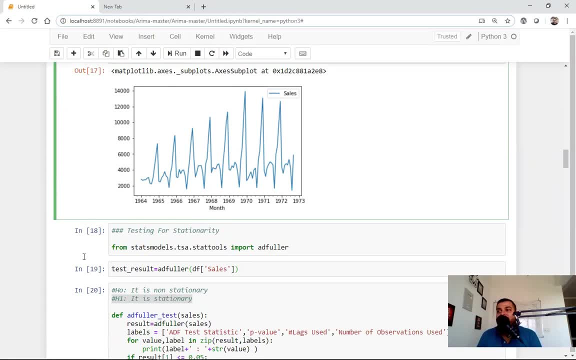 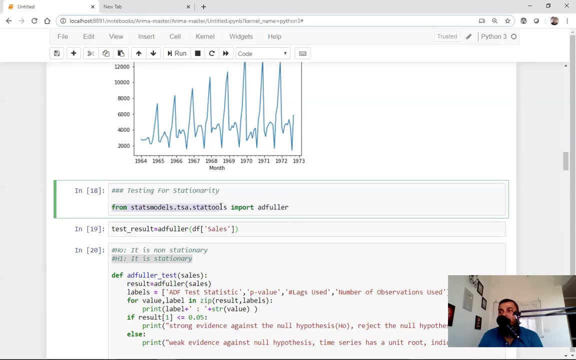 variance or whether it is almost same. so we basically apply something called a Dickey-Fuller test. okay, so Dickey-Fuller test is basically imported from stat models, dot, TSA, dot. stats tools, from import that I'm going to import the ad fuller. now, when I'm importing this ad fuller, all I have to do is that I have. 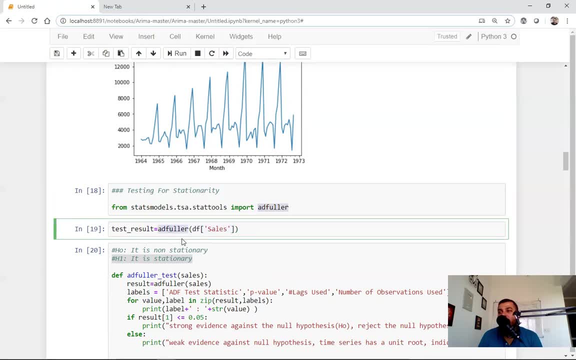 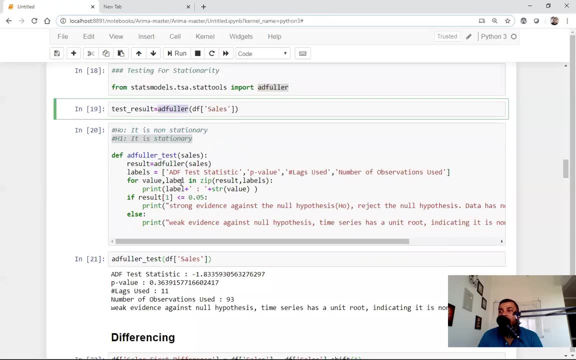 to give this whole data BF of sales into my ad fuller function. now, ad fuller actually gives us five different values, okay. the first value: we basically say it as ADF test statistics. the second value: we say it as a P value. the third value: we say it as number of lags used. the fourth value: we basically say it as number of. 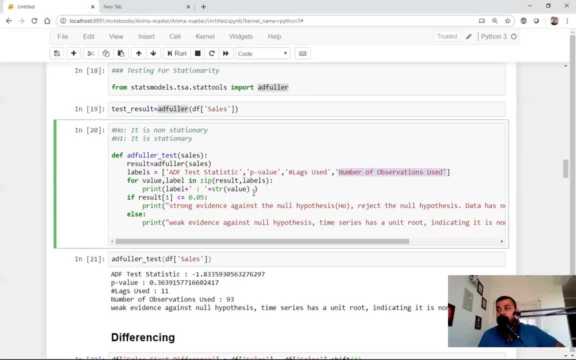 observation used now understand over here. the most important thing that we require is P value. and how does Dickey-Fuller test work? Dickey-Fuller test is again a kind of hypothesis testing wherein the null hypothesis basically stays- says that the data is not a stationary. 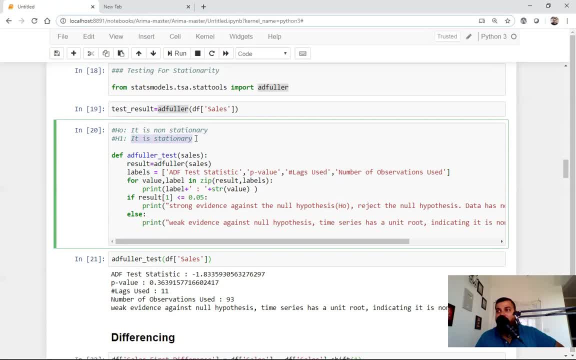 okay, whereas my alternate hypothesis says that it is stationery. so, based on this particular condition, if my P value is less than 0.05, it basically says that data has no unit root and and is stationary. so that basically means that if we are getting 0.05, we are rejecting. 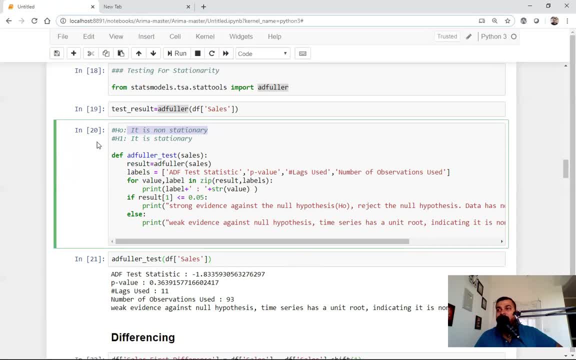 the null hypothesis? okay. and if you are rejecting the null hypothesis by default, the alternate hypothesis will get selected. that is called, as it is stationary. and if you don't know about null hypothesis or alternate hypothesis hypothesis, please go check my videos. I have explained everything about it, okay. 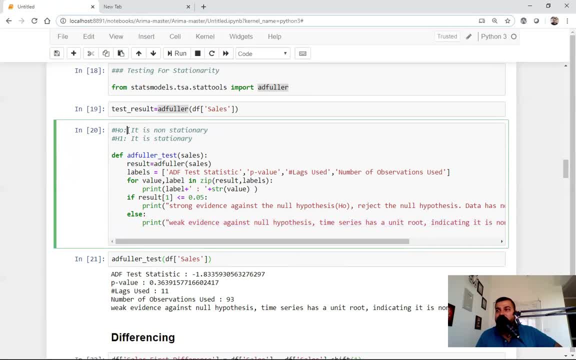 and similarly in the else block, I'll say that it is not stationary at that. at that specific time the null hypothesis becomes true. so every information has been given. what I am doing over here, I'll just go to this particular code. so in the at fuller, I'm providing the data of the sales. okay, and this is just a. 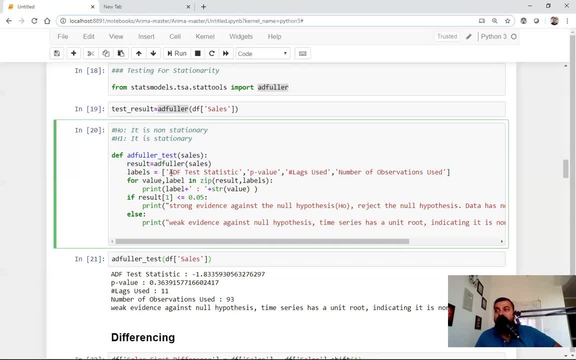 function. okay, function now. this will result five different values like this, so that all values will be present inside result. I'm just doing a zip over here. zip basically means that I'm combining whatever result values are there and this particular label values and I'm checking that if that particular 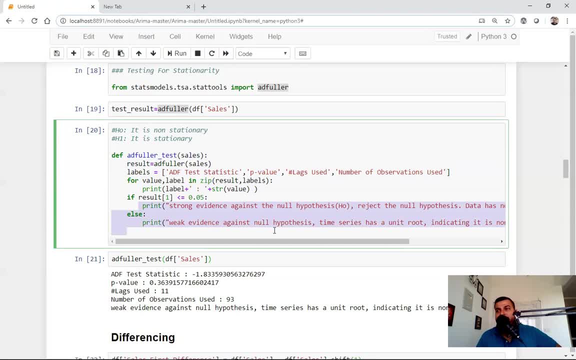 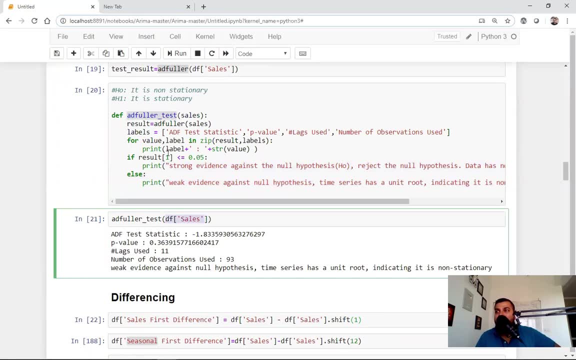 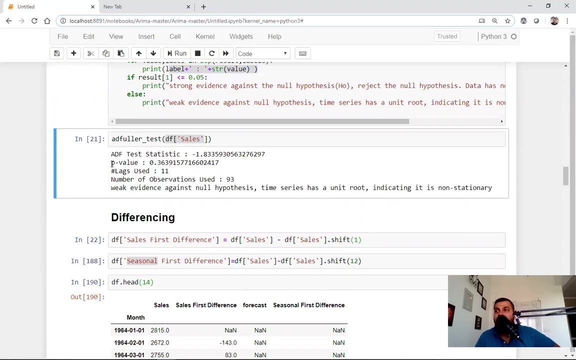 value is less than 0.05. and then this is pretty much simple. now, whenever I call this particular function, you can see that I'm giving BF sales and I'm printing all the labels and this particular value, so I'll be getting ADF statistics like this, like this, like this. now, here you can see that clearly, my P. 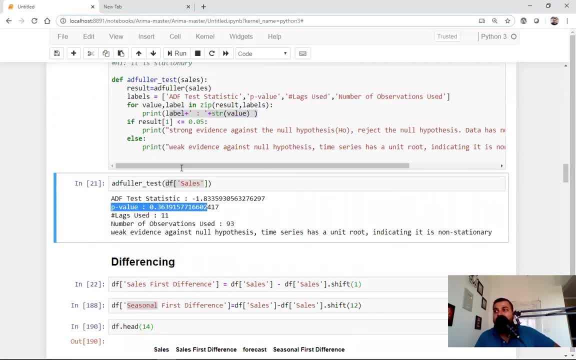 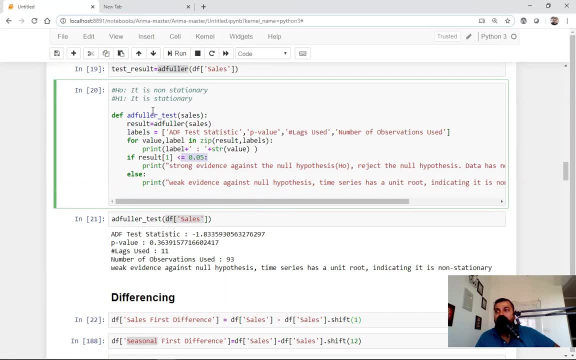 value is 0.36915, okay, which is not definitely less than 0.05. if it is not less than 0.05, what are we are going to do? we are going to reject the null hypothesis, because my null hypothesis says that it is non stationary. okay, so 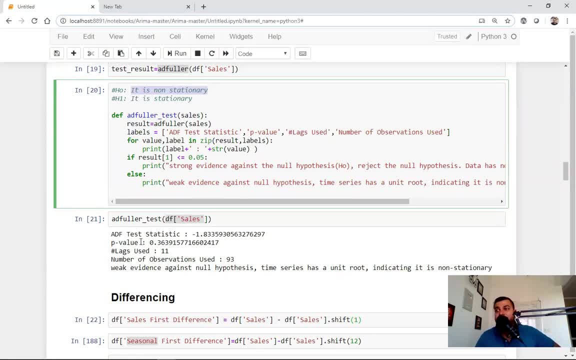 we are going to reject the null hypothesis and still, that basically indicates that my data is not stationary. okay, sorry, we are not going to reject, we are going to accept the null hypothesis because it is less than 0.05, but over here this particular value is greater than 0.05. okay, so we are. 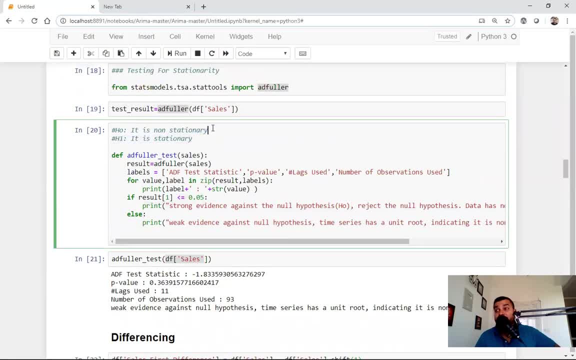 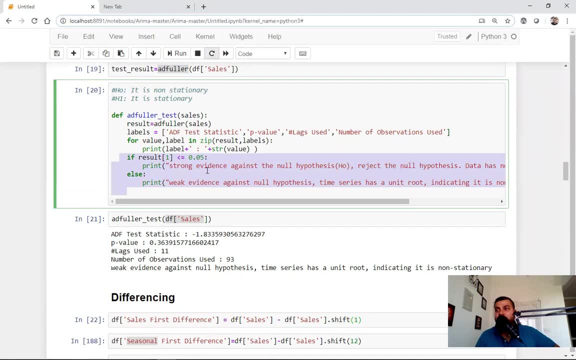 going to accept the alternate, sorry, and we are going to accept the null hypothesis saying that it is non-station. just see this particular condition, okay, and there may be some confusion. so make sure that you always, you know, work with this particular function. so when you are passing through this particular function, 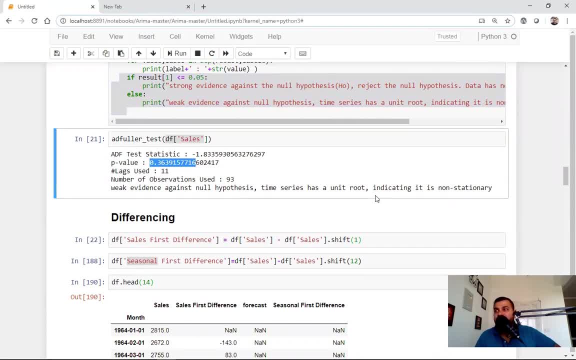 and getting this particular value. weak evidence against null hypothesis time series are indicating that it is non-stationary. now, now is the most important step. if the data is non-stationary, what do we do to make it stationary? now, there are two things that we can actually do. okay, the first thing: 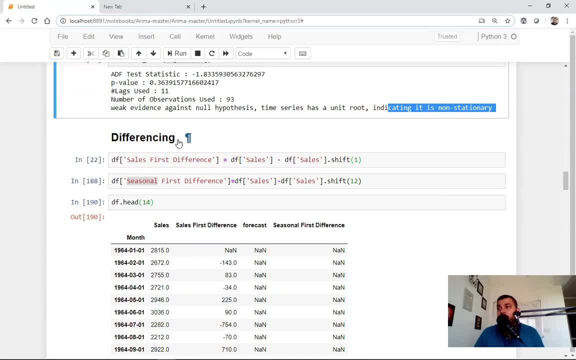 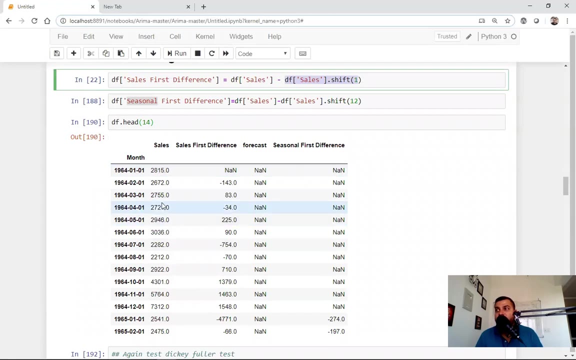 is that, guys, we have to do something called as differencing. now, what does differencing actually mean? now, in differencing, what we do is that we just shift one position, okay, one position of that particular sales data. now see if we are pushing, if you are shifting one position, okay, if I, if I just say what is. 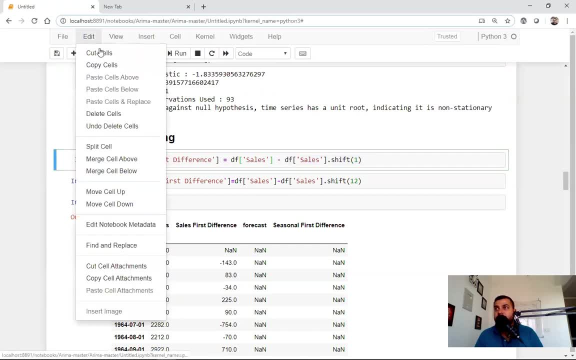 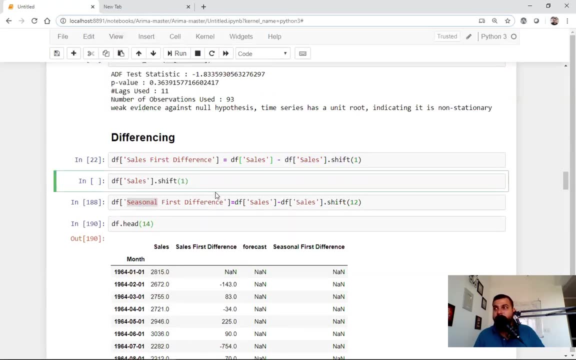 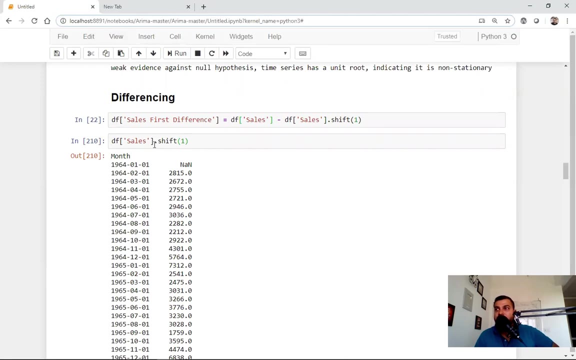 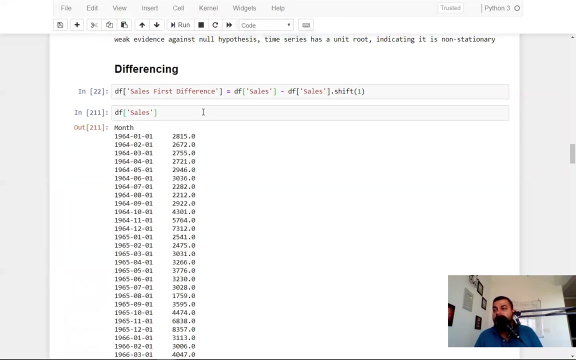 the shift of this. okay, let me just show it to you now, if I just paste it over here. okay, if I say shift of one, now here you can see that one position it will be moved down. initially my records are looking something like this. initially my records look something like this: okay, now what I'm 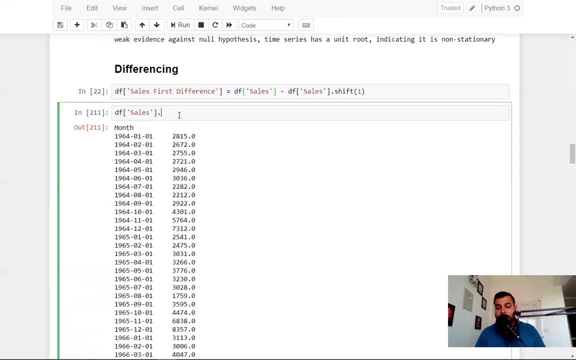 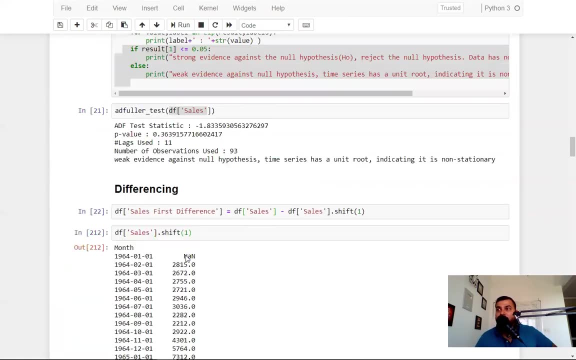 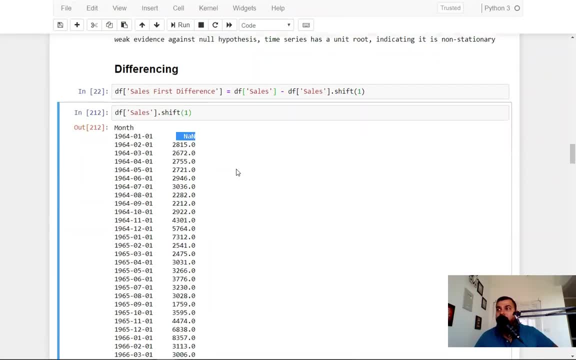 position put it down, and this will be initialized to nan value. so what I'm going to do is that, if I want to find out the first difference, I'm going to subtract D of of sales with D of of cells, dot shift of one. now, when we 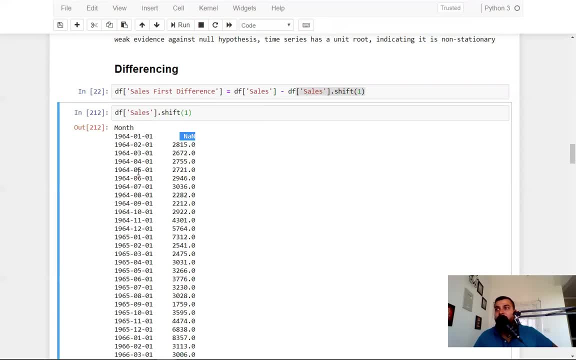 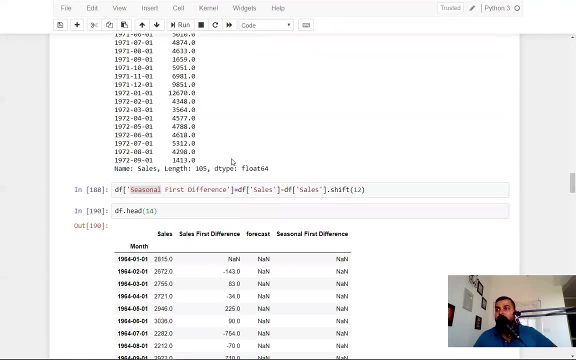 subtract the first values, man then obviously after subtracting also will be getting man. so here you can see that when I am actually trying to create a new column called a sales first difference, here you will be able to see that I'm getting a nan value and all the differences over here. okay. 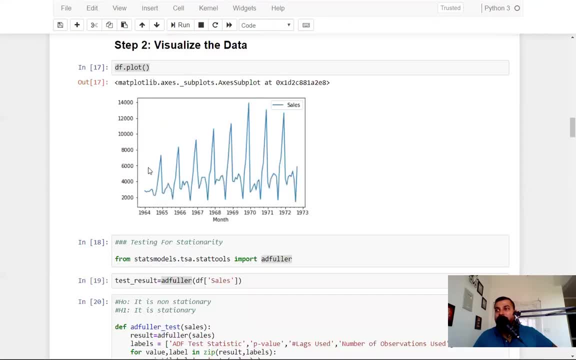 but remember, guys, I told you that my data looks seasonal. right? so if my data looks seasonal, I should not just be subtracting by shifting just by one position. if my data is not seasonal, at that time you know I can do that okay. but here the main thing is that my data is seasonal and based on this seasonality. 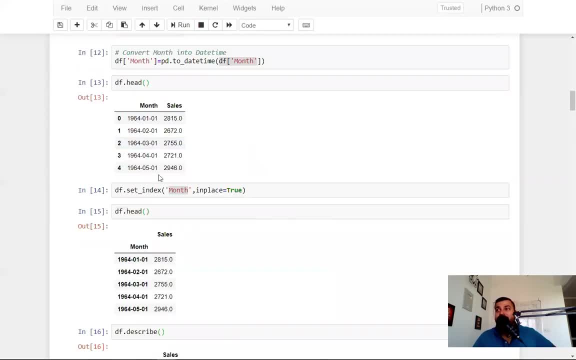 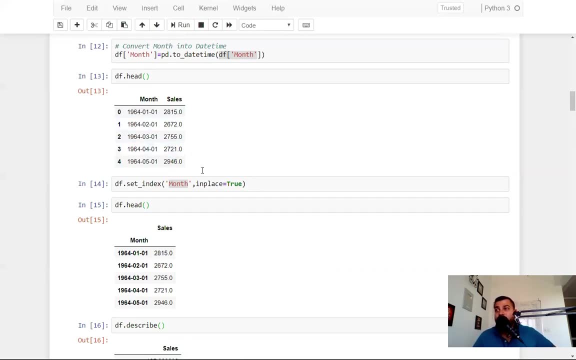 of the data, the time that is taken over here is basically two months, like one year has 12 months, right, sorry, not to 12 months. so one year has actually 12 months. so here we can see that the data from here going up and again coming down. 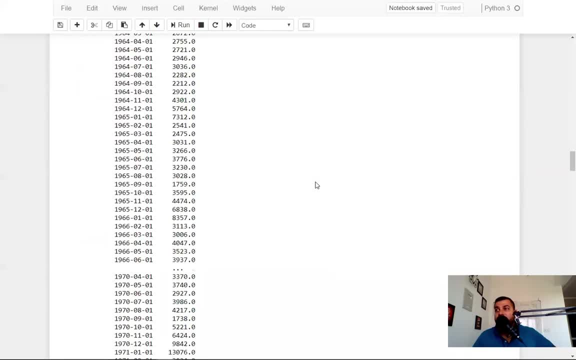 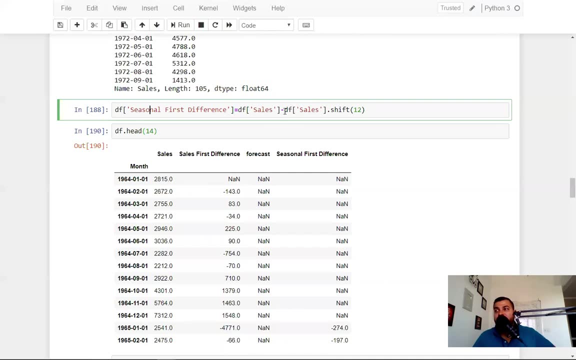 is basically one cycle of 12 months. okay, so for that we, instead of doing just a single shift difference, we do something called a seasonal difference. a seasonal difference basically means that here, instead of shifting by one, we'll be shifting by 12. okay, so, when we do the shift by 12 and when we find out, 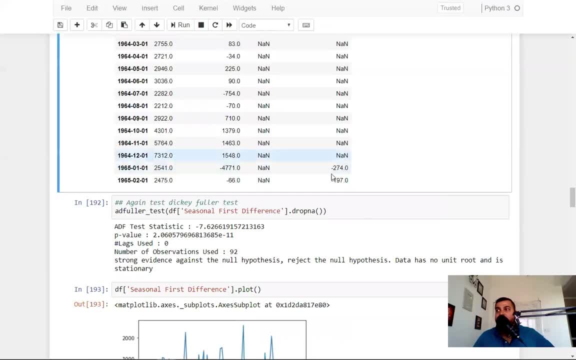 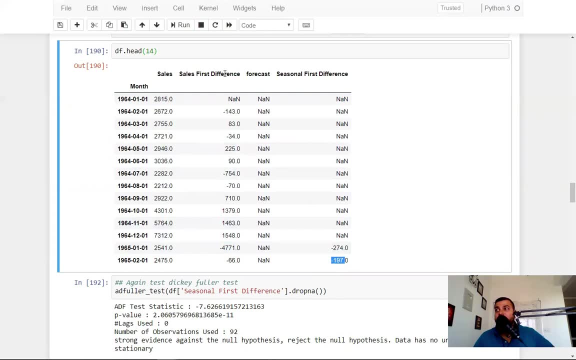 then we'll be able to see this particular seasonal first difference. okay, so this is how it will look like now. remember, in the seasonal first difference also, I have so many nan values. now, after doing this, what I'll do is that I take this particular data and again test it with my Dickey Fuller test. 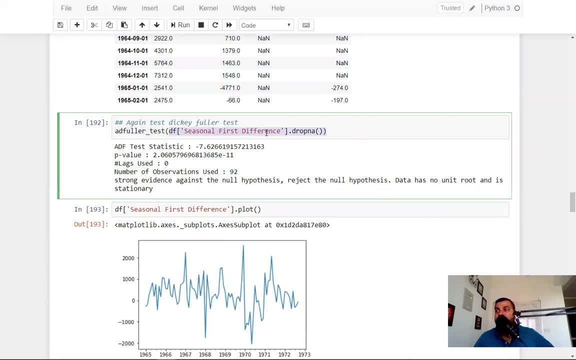 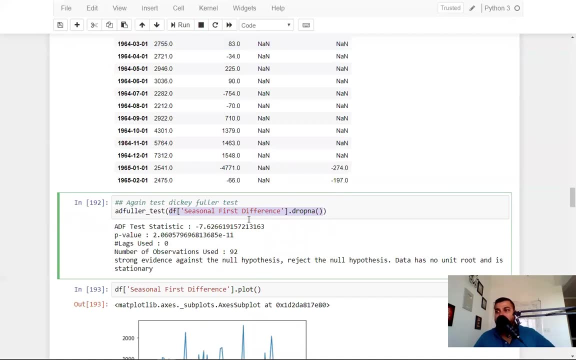 okay. so here I'm again taking my ad fuller test. I'm passing this particular information. make sure that you pass dot drop in it, otherwise if this na value is there, it won't work well, it will give you a lot of errors. now, here you can see. 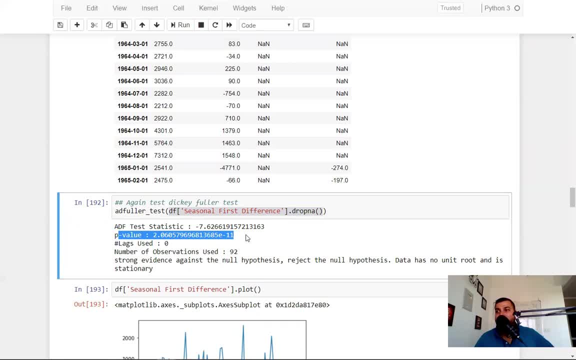 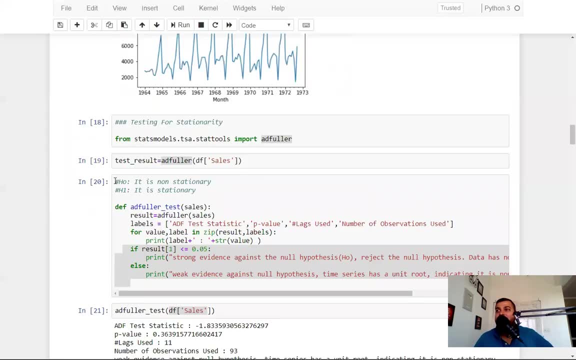 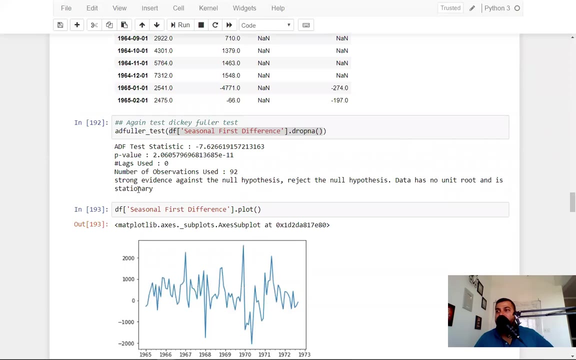 that you are getting your p-value less than 0.05. okay, now you can basically say that your data, the data, is stationary. now, what you are doing over here, you are actually rejecting the null hypothesis, accepting the alternate hypothesis. now, finally, you will be able to see this particular information now if you go and 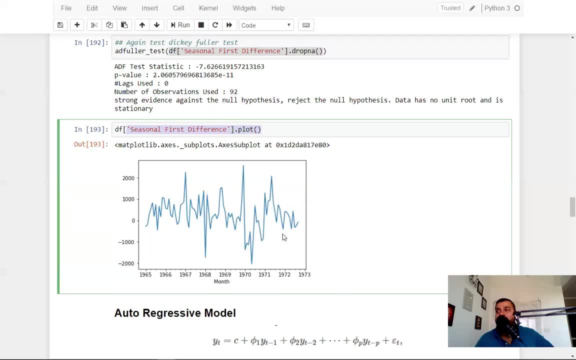 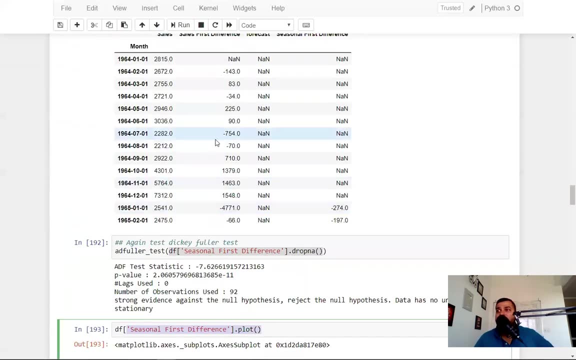 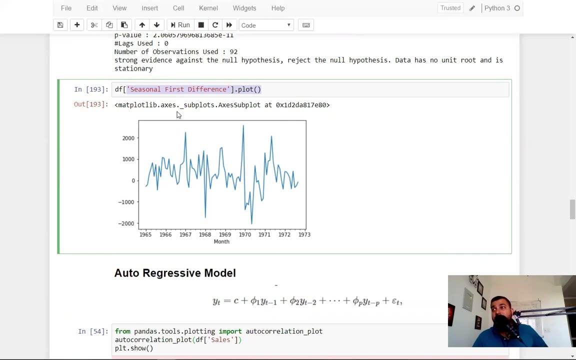 see your seasonal first difference dot plot. it looks almost stationary. now, yeah, this data almost looks stationary is? there are small variance, so we are taking the p-value as point zero five. if this was exactly zero, then that would have been a wonderful stationary graph. okay, so now? 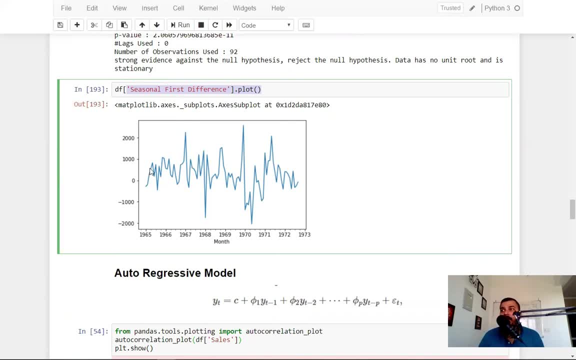 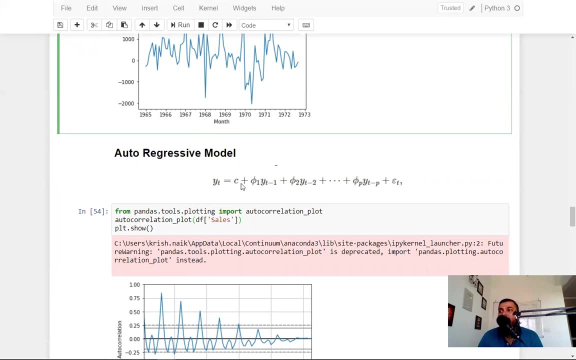 we are. we have to stop away. once your data becomes stationary, we have to stop away now. what does auto-regressive border basically say? so this is my formula of the auto-regressive model. like, Y of T is equal to C plus 5, 1 plus. 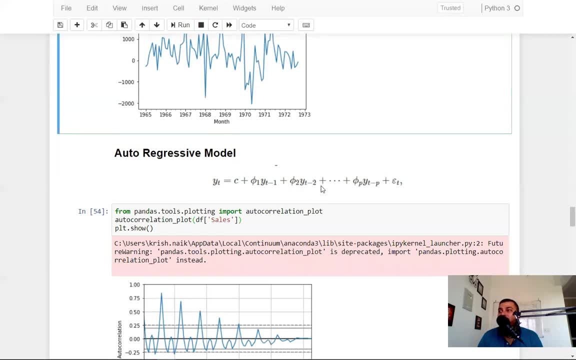 YT minus 1, like this, this: these are lags: T minus 1, T minus 2, T minus P. then how many data do we have to take, suppose, if I want to predict the sales of today? okay, how many previous data I have to actually consider? and that can be only. 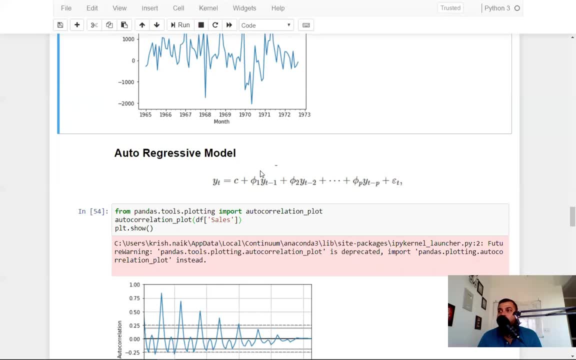 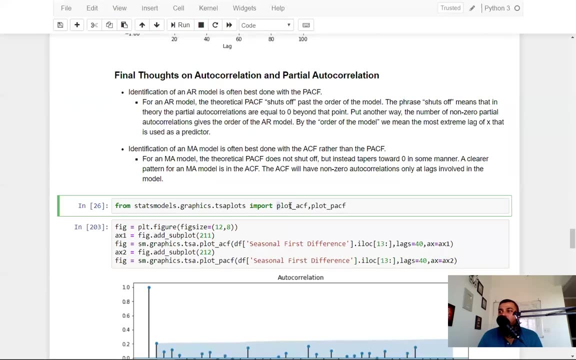 done by something called as auto correlation plot. okay, so there are two things, just don't worry about this particular graph. we have to use something called as autocorrelation and partial autocorrelation, and these are presents inside this particular library, called as statmodels, dot, graphics, dot. 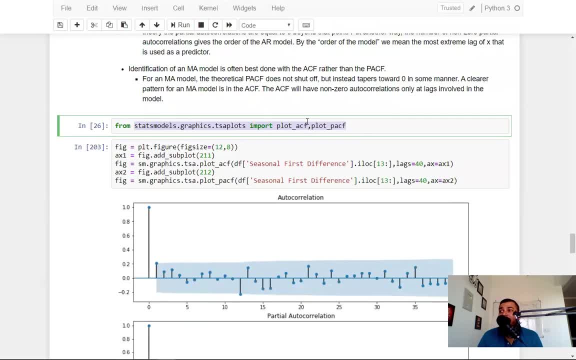 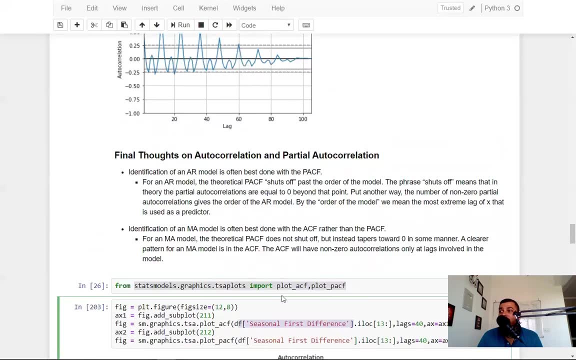 TSA plots. import this particular values. now for selecting this guy's, for selecting this again, we will be passing our seasonal first different data, not the whole data set, and remember what this particular value is saying. we this particular value saying that, whether we have to take till YT minus 2 or whether 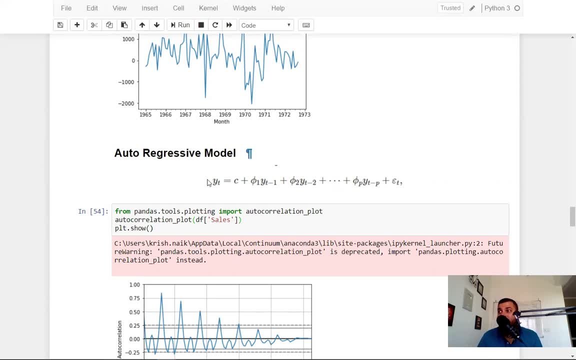 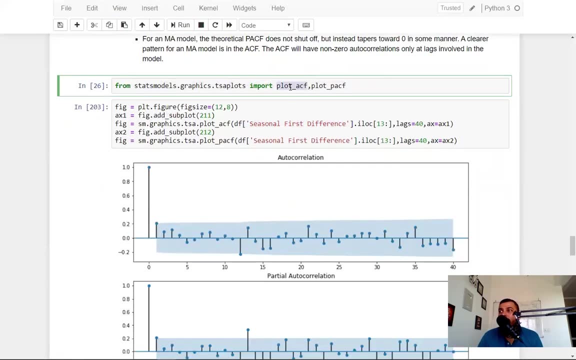 we have to take till YT minus 3, so that particular formula will get set right and, based on that, the forward forecasting will be done. now, in order to do that, what I'm going to do is that I'm going to implore plot underscore ACF. 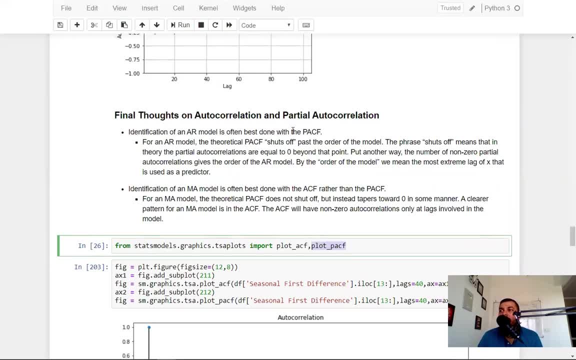 plot underscore PS here. one thing that you have to note from this particular description, which I have actually given identification and again I'm told you, Arima has three components. one is autoregressive, one is, you know, the middle one, which is called as differential, differencing. the third one: 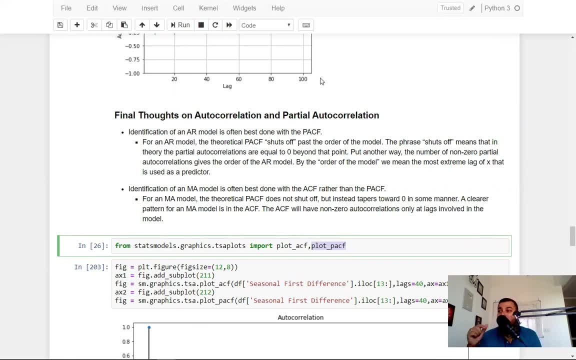 is called as moving average, okay, so differencing, also called as integrated. now, first of all, we need to identify a our model. okay, so identification of an AR model is based is often best done with the PSCF. PSCF is nothing but partial autocorrelation, partial autocorrelation. 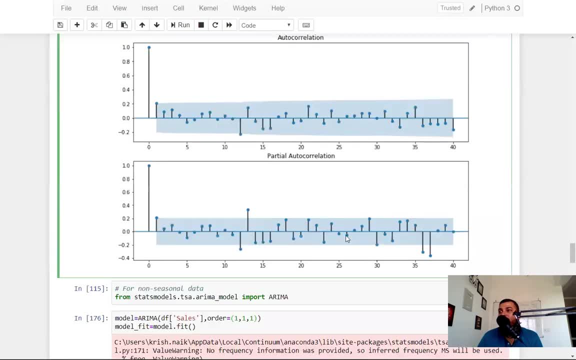 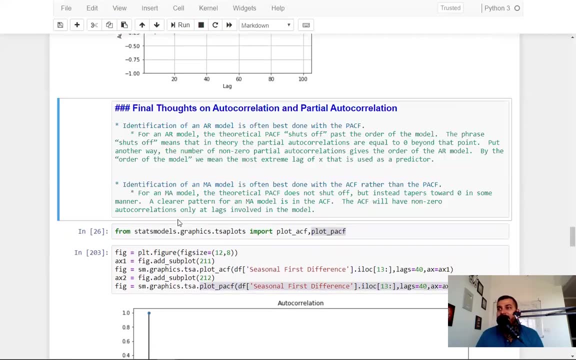 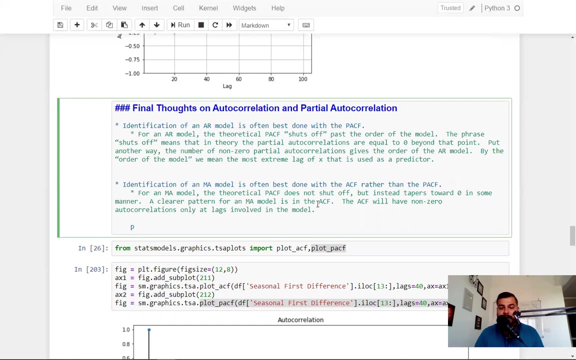 is happening because of this particular code. now, here you can see that particular code. okay, now, if I want, if I want to find out the AR, and usually what we do is that we select three values. guys always remember, in our Arima model we have to give three values: P, Q, sorry, P, comma, D, comma, Q. okay, so P actually. 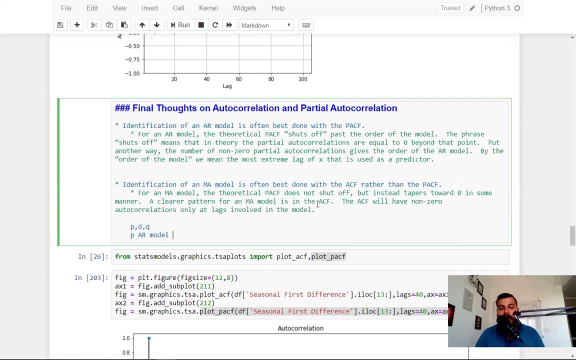 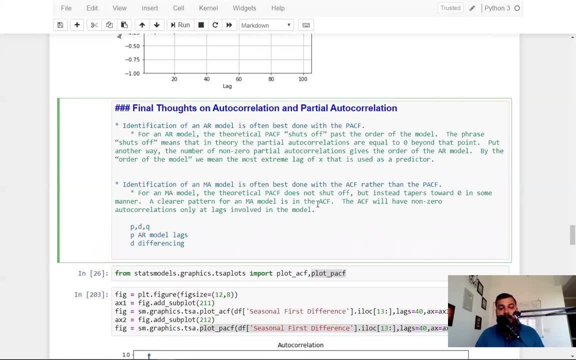 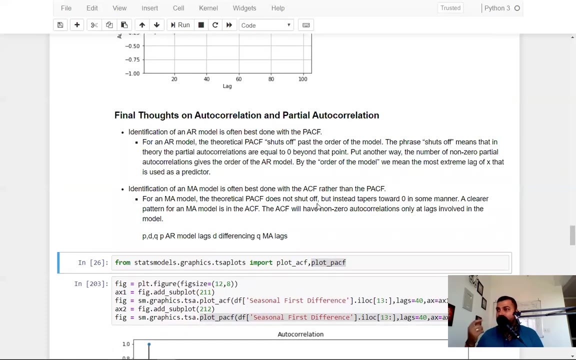 specifies about my AR model lags. AR model lags, okay. D is difference in D is differencing and Q is moving average lags- okay. so these all are the values that we will be considering or making finding out. okay, we need to specify these three values always, remember. okay, now we were talking about. 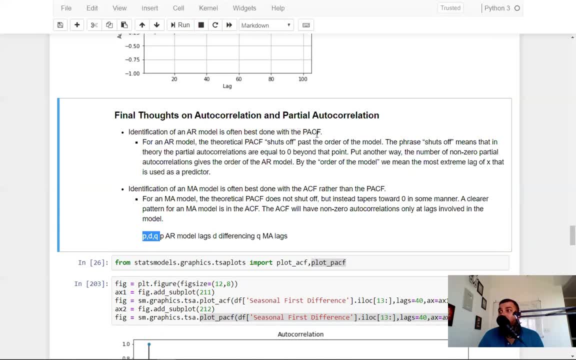 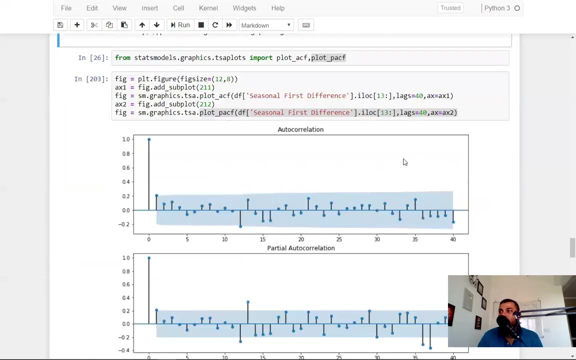 the AR model. so AR model is oftenly best done with PSCF, that is, partial autocorrelation. now remember, in this particular point, for an AR model, the theoretical PSCF shuts off past the orders of the model. now what does this shuts off mean? understand, guys over here when I am actually and remember when I'm. 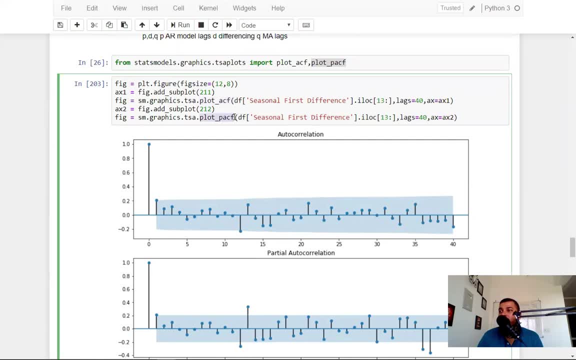 calling plot ACF. this is for autocorrelation. plot underscore PSF is for partial autocorrelation. the data that we are giving is first, seasonal, first difference, and remember why we are giving I log 13 colon because remember the first two L records are nan values. I can also give dot drop any. okay, you can. 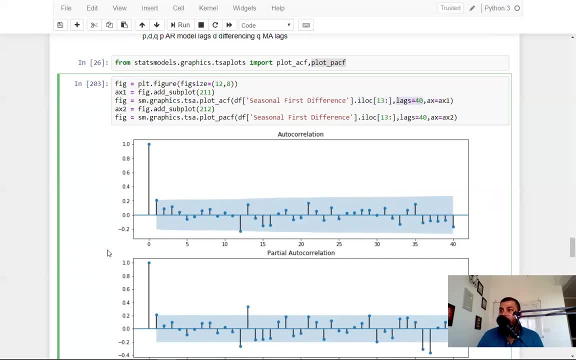 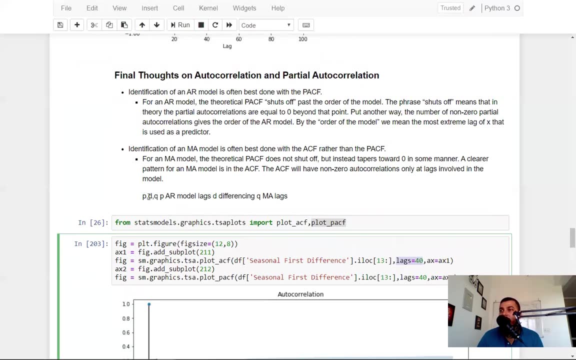 give any of them and the total number of lags that I want to see is for 40, then I will decide that how many lags I have to consider for AR, how many lags, that is, what should be the P value, what should be the key Q value, what should be the D? 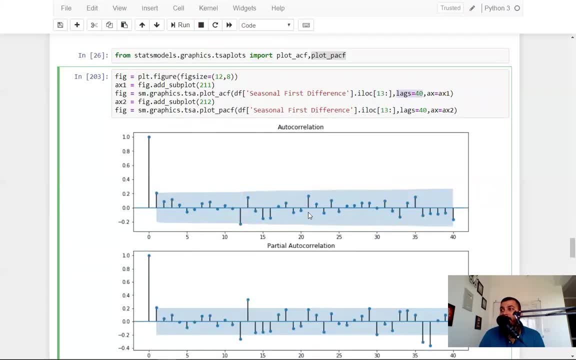 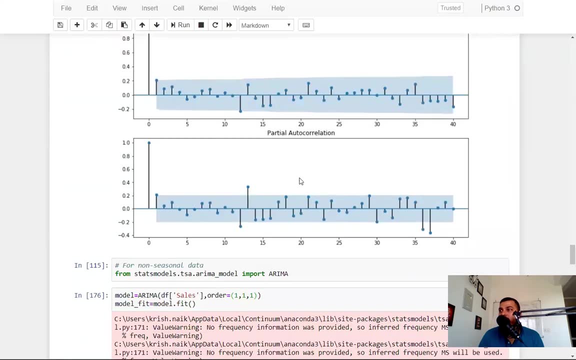 value. now one thing that I observe from this particular graph and remember: first of all, I need to check my AR model. it is best done with PSCF, so I will go with PSCF, and we have also noted one points which is called a shuts off, shuts off. 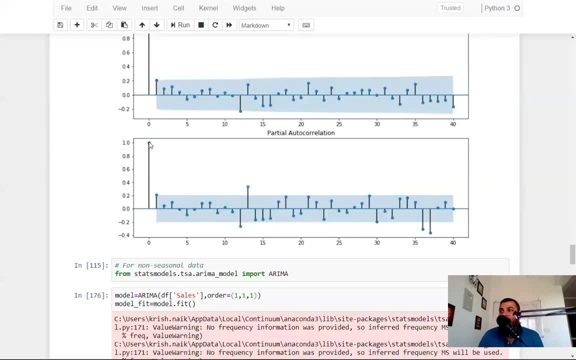 what does it mean? remember, in this first case it is very, very high. in the second case it has come down, there is some correlation, and then in the third case it has just been like below the zero and zero point two right. so here the sudden shut down or shutoff is actually done. there is sudden 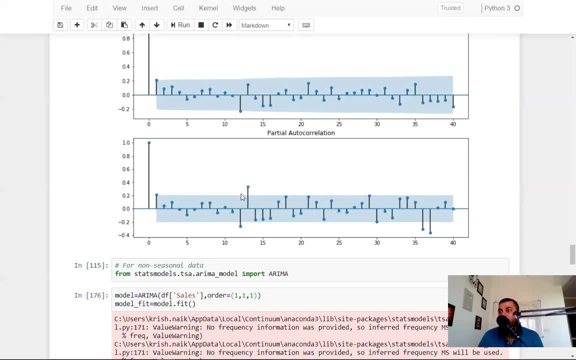 decrease and it is all near to zero. okay, after this particular point, you can see that there are some values that are coming up, but it is fine, but remember, from here to here. then suddenly it is coming over here, right? so we should actually note down this particular point where it. 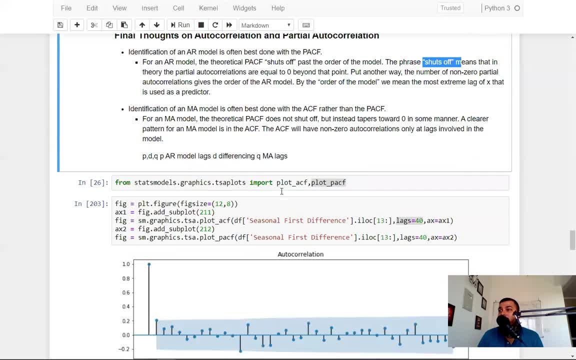 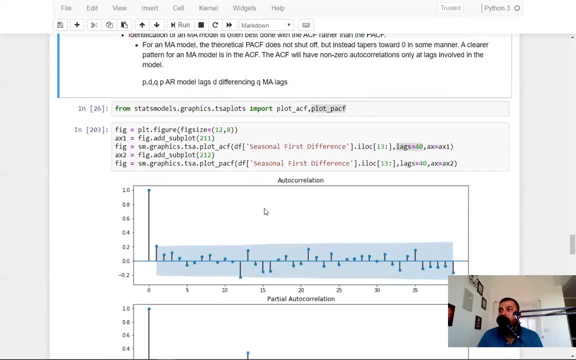 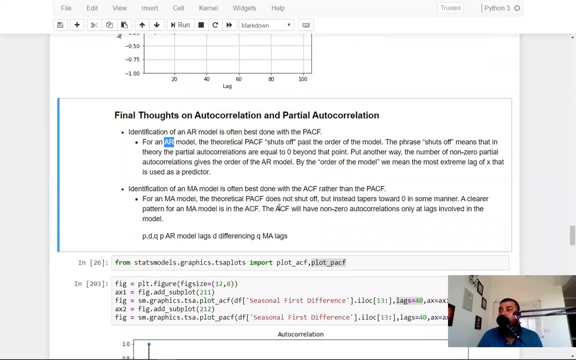 this particular point is for one. this one should be the value of AR value. okay, AR value, so that basically means my P will get initialized to one. now the knowledge. next thing is that what should be the Q value? now, for Q value is basically my MA model- is often best done with the ACF rather than the PCF, and it 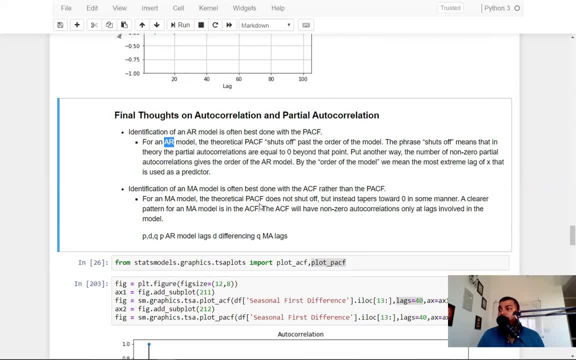 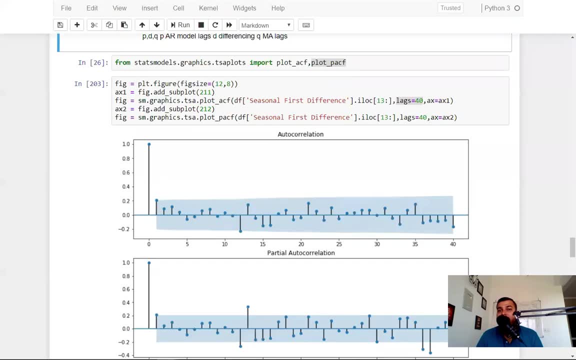 accepts. it accepts that the theoretical PSCF does not shut off but instead tapers towards zero. now this, this basically means that guys, usually in PSCF- I'm just going to draw a graph, you know, so that will be easy for you to understand- it does not shuts off like this suddenly. okay, it will be having an. 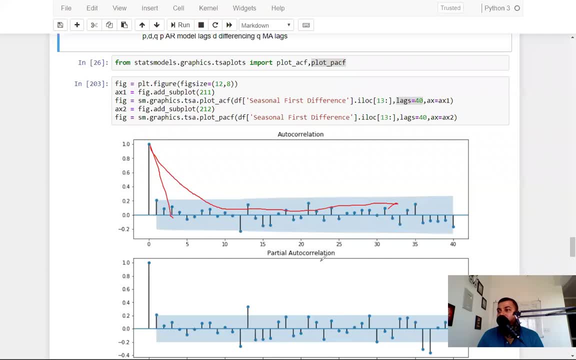 exponential decrease like this, whereas in this particular case, in partial autocorrelation, it will have sudden shut off, shut down like this, okay, and then it'll it'll be mingling over here itself, okay, but here we'll be having an exponential decrease like this. but here, in this particular case also, we 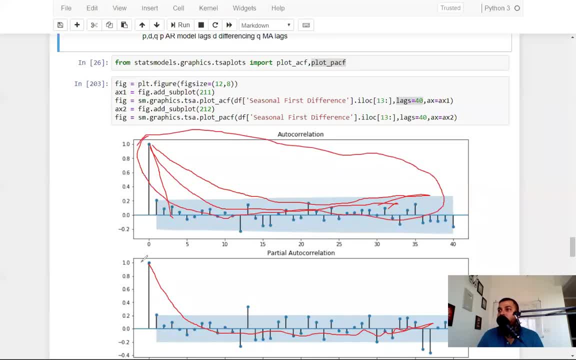 don't see any exponential, exponential decrease, right? so what I'm going to do is that I'm just going to consider autocorrelation as zero in this case, because here we are focusing more on AR value. okay, AR value, but again, if you just take one value also, because till one it, you can see that there is an. 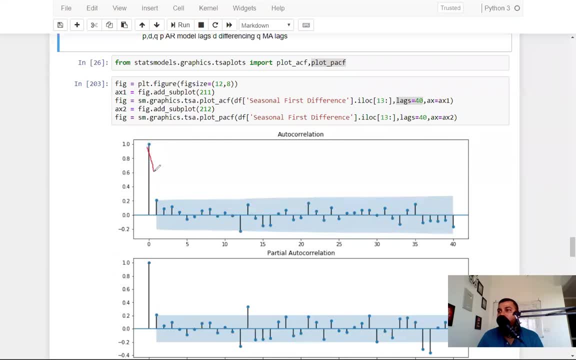 exponential decrease. right, see over here till one. there is an exponential decrease, but after that it is just juggling around, right. so here and here you can see that it is sudden decrease till one also. okay, and then they are values tingling over here. okay, so this is. 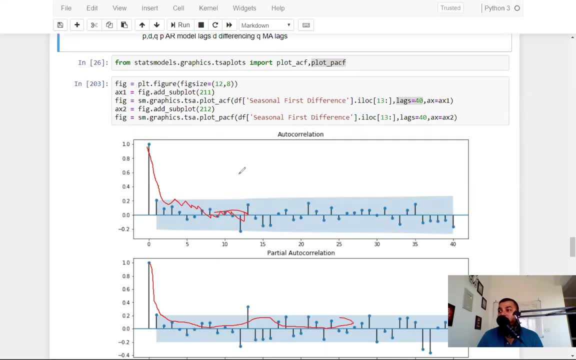 called a shuts off, and for the autocorrelation where we are checking for MA, we should check whether there is an exponential decrease or not. but here the exponential decrease is till here, okay. after that it is not there. here the shutdown is still here again. so what we can do is that either we can select my 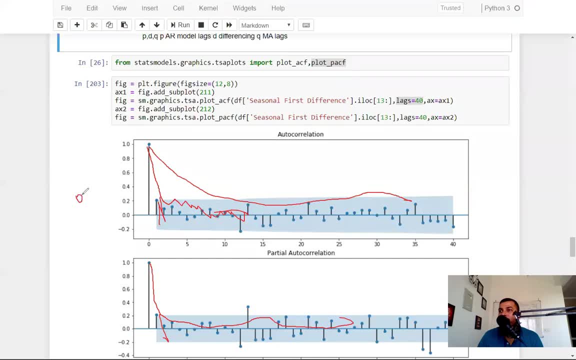 autocorrelation value, that is, my MA value as zero or my Q value as zero, okay, or my P value. P value will definitely be one, okay, I can also go with Q is equal to one because the exponential, you know the exponential, if I see over here, this particular value is decreasing exponential only till here. 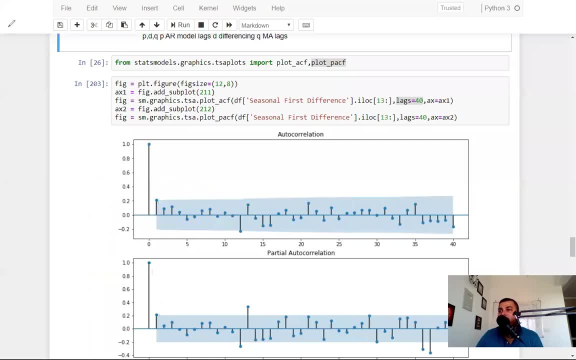 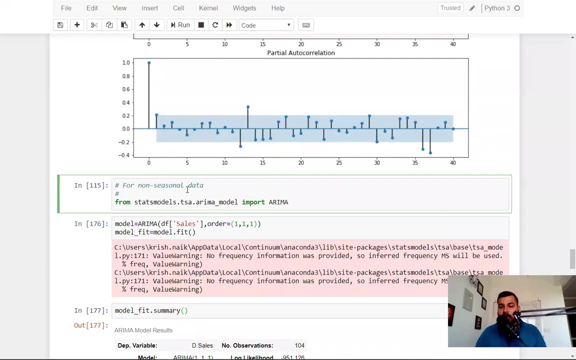 at this particular point, which is my one. okay, so what I can do, I can take zero or one, but I tried with both zero and one and, trust me, one also work well. okay, now I am going to set my D value as one. okay, so I am going to set my D value as one. 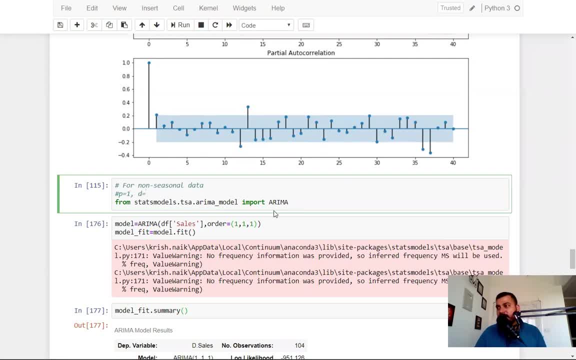 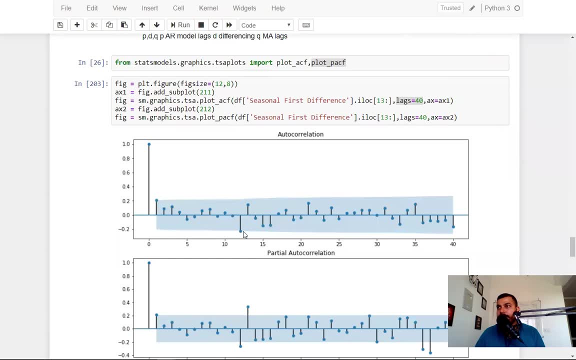 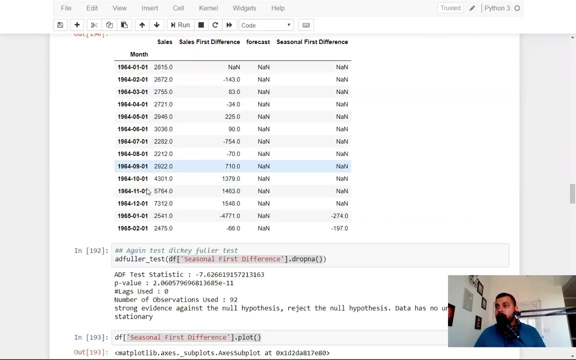 once we are able to find out what we have done over here. we have actually selected of P value, so my P value is equal to one D value. also, is remaining guys, how many seasonal difference differencing? we did, okay, seasonal differencing only one time. we shifted, so I'm going to set my D value as one, okay. 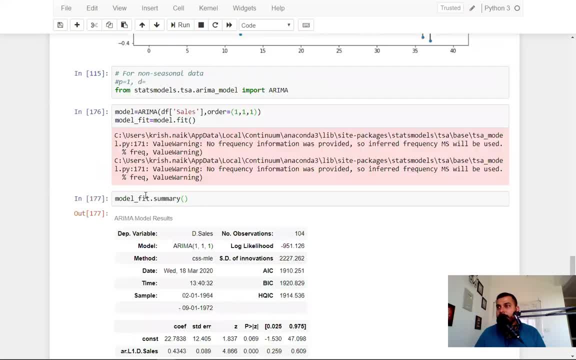 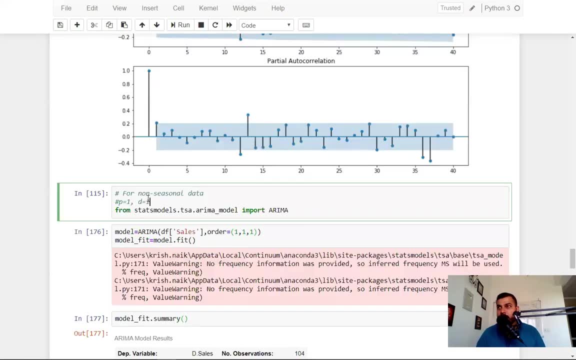 so I'm going to set my D value as one. oops, where is it? oops, it's going very fast, just a second. okay, I'm going to set my D value as one, okay, and then I've already selected my Q value as zero or one, I can. 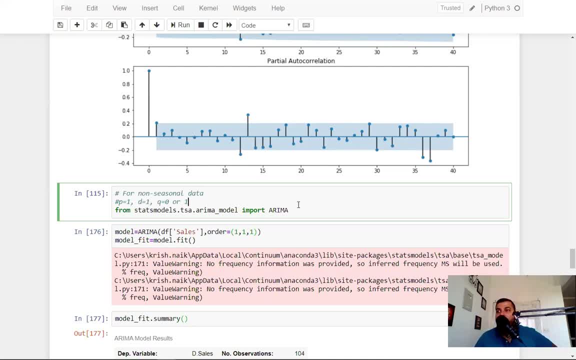 check it either with zero or one. now remember when I am implementing Arima. I told you that Arima should be selected only when your data is not seasonal. but in this particular case, data is seasonal. but I wanted to show you how you can implement Arima models. I have given this. you have the F of sales. 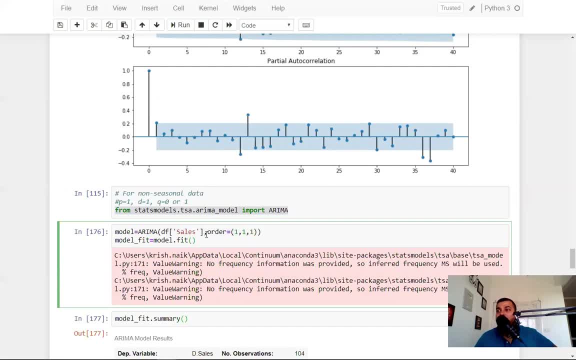 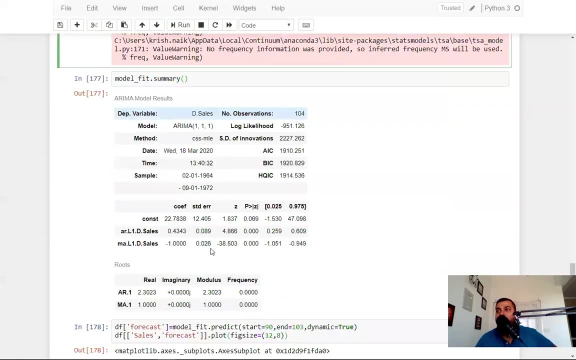 order: 1 comma 1 comma 1. remember, this order is nothing but P, D and Q. okay, you can either use 0 or 1, but since this is seasonal data, this will not work well, because after this, when you are seeing the forecasting, it looks something like: 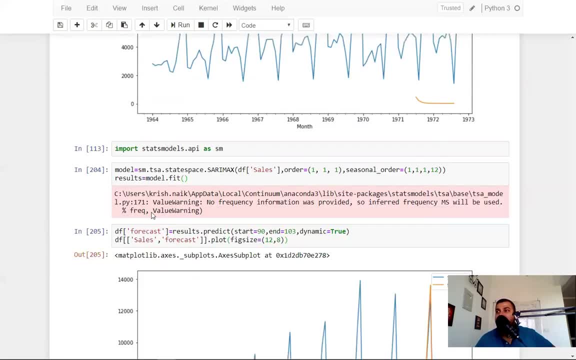 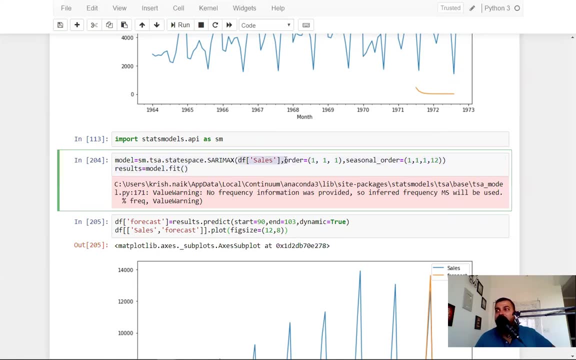 this, so don't focus on to this. I'll be showing you the exact way how we should do it. so there is something called a seasonal Arima X. so here it will be requiring D- F of sales. the order value will be P- D and Q: 1, 1, 1, 1 either you. 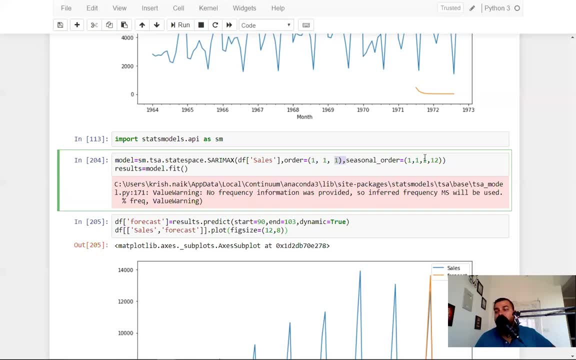 can use 1 1 1 0 or 1 1, 1, 1. I saw that 1 1, 1 was working well. my P value should be 1, my D is 1 and my Q can be 0 or 1, and there is one more additional parameter. 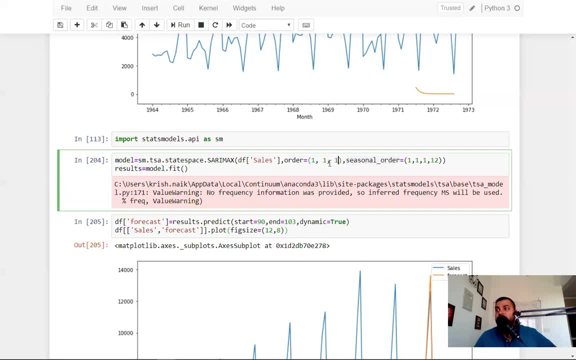 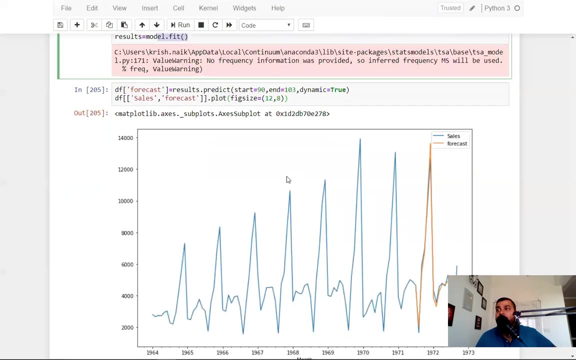 which is called a seasonal underscore order. in seasonal underscore order the P Q- D will be the same value, P D- Q. but this 12 basically says that in and season by how many number you are actually shifting? that should be the value over here. so here I've actually given as 12, then I do model dot fit. okay, then what? 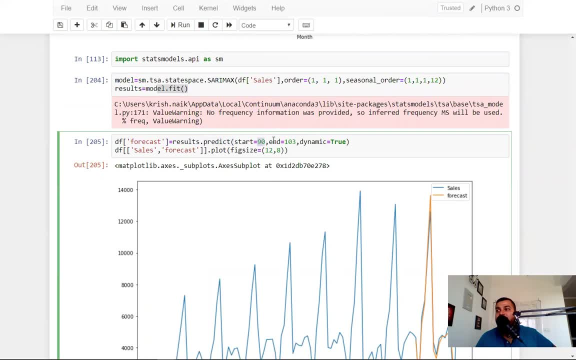 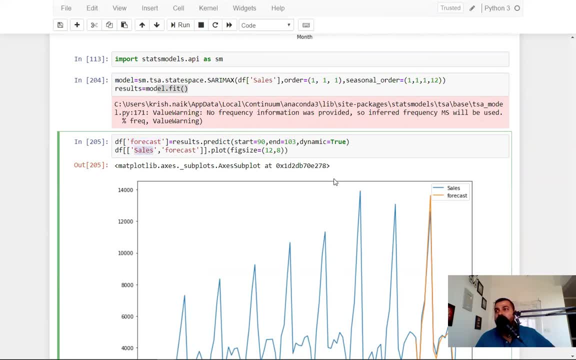 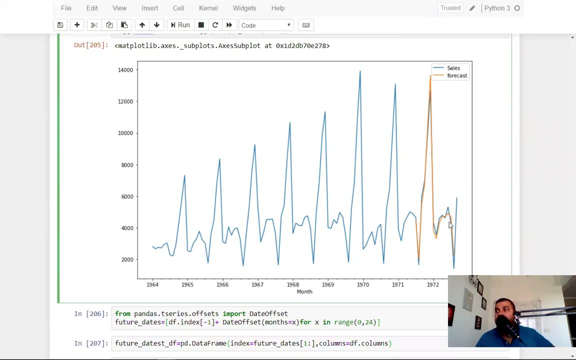 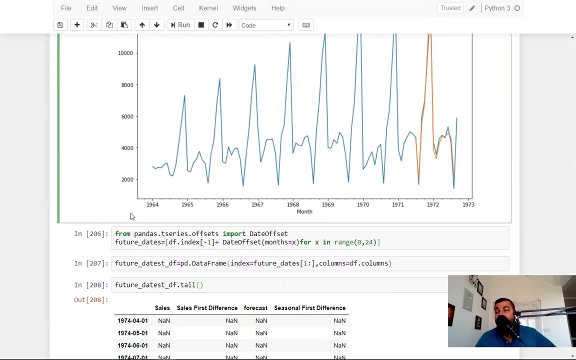 okay, consider that as an forecast column and try to plot that particular column like here. you can see that the blue line is my real data and my forecasted orange line is my real data. sorry, in my predicted data it looks good, but still I need to find out how will be the future prediction? prediction or 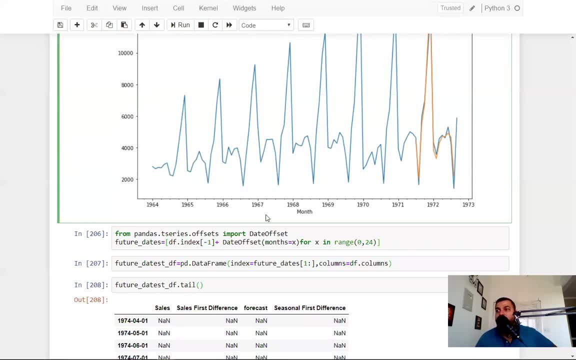 projection looking like, or how will be the future forecasting looks like. okay, I So for that, what I'm going to do is that I'm going to create some additional data set for 24 months, And for that I'm just going to use simple pandas by importing the data offset.